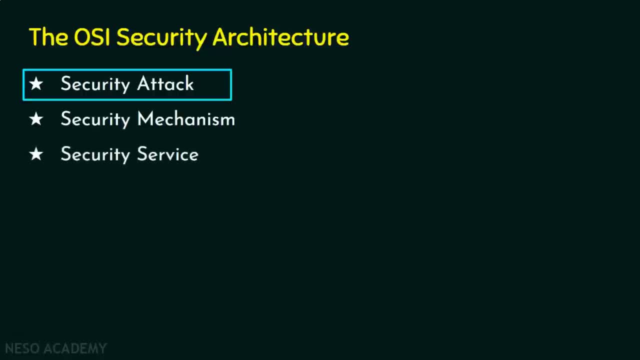 mechanism and number three, security service. In today's lecture we are going to focus on security attack. Let's dive into what is security attack. We know attack is an action that compromises the security of an individual or an organization and, if the attack is successfully launched, 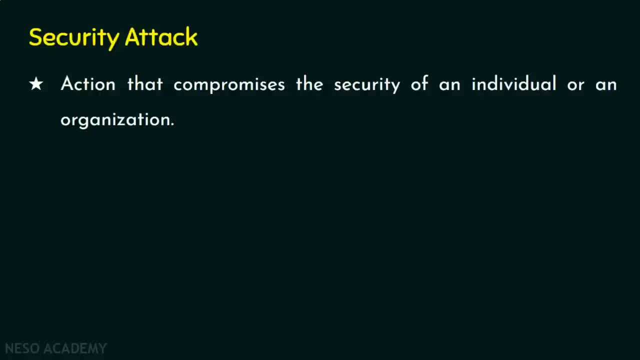 then the effects of the attacks would be loss of data or corruption of data or ransomware attacks or injection of viruses, swarms or malicious softwares into the network or defacing the servers, and many effects are possible. The attacker only knows for what he has launched the attack. 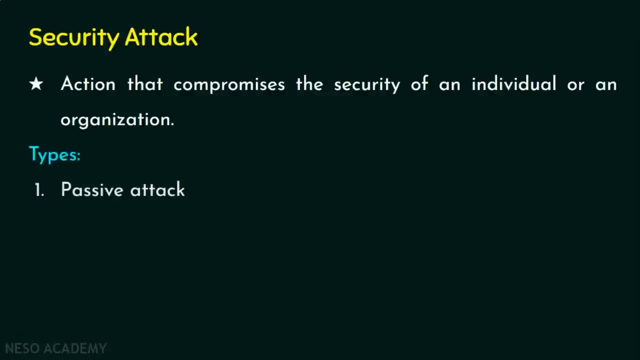 and this attack is basically of two types: Number one, passive attack and number two, active attack. Firstly, we will see about passive attack. Passive attack attempts to learn or make use of information from the system. Basically, passive attacks are unauthorized reading of messages and no modification. 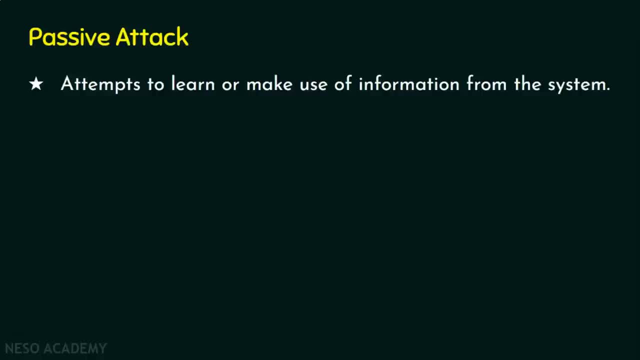 of messages involved. Suppose if there is a sender and a receiver. If sender is sending some data to the receiver and the attacker's intention will be just observing or reading what message the sender is sending to the receiver- and that's why I quoted passive attacks- are unauthorized reading of. 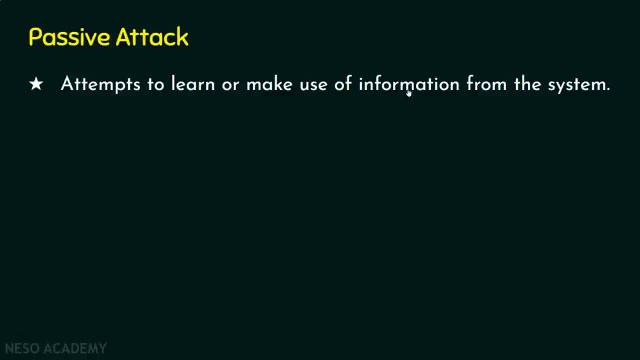 messages and this attack is mainly to learn or make use of the information from the system and not affect system resources, because the intention of this attack is just seeing the message content. Obviously, this attack will not affect system resources, As mentioned the main motive of the attacker. 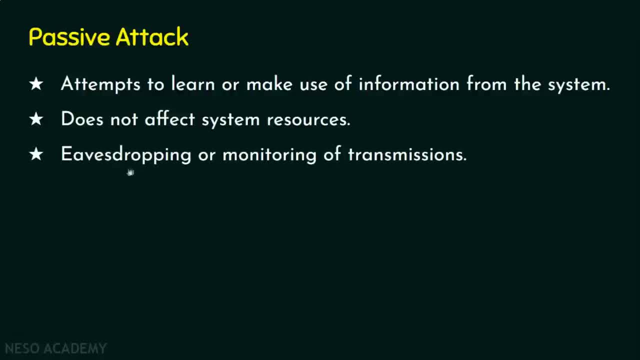 is just to observe or eavesdrop the conversation, and this point says that this attack is mainly eavesdropping or monitoring of transmissions. Whatever the sender and the receiver are transmitting, the attacker's intention will be either eavesdropping the messages or monitoring what kind of 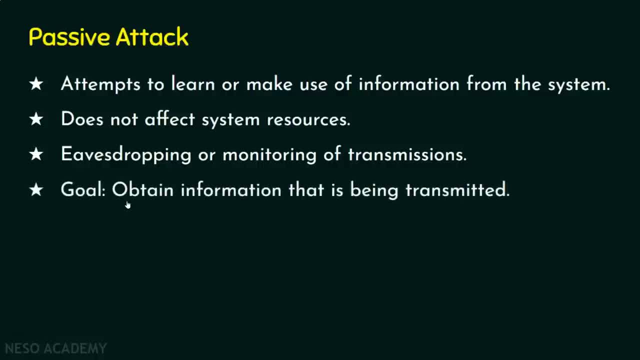 transmission is taking place. So the goal of the passive attacker is to obtain information that is being transmitted. Let's see the two types of passive attack. Number one is release of message content and number two traffic analysis. So before seeing the examples, we must understand one thing: that in passive attack, 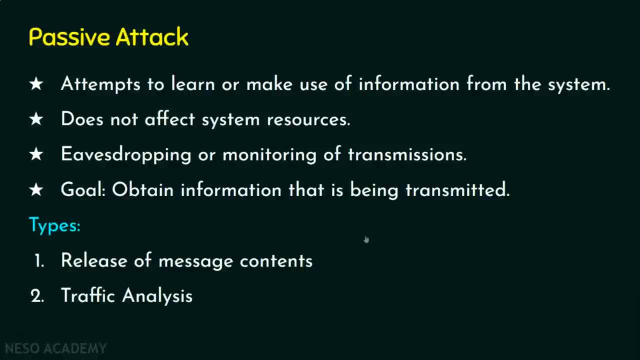 it's just unauthorized reading or monitoring the messages. Let's assume there is a confidential telephonic conversation or a confidential email is being transmitted. This attacker's intention is just to know what is being transmitted. So the goal of the passive attacker is to obtain information. 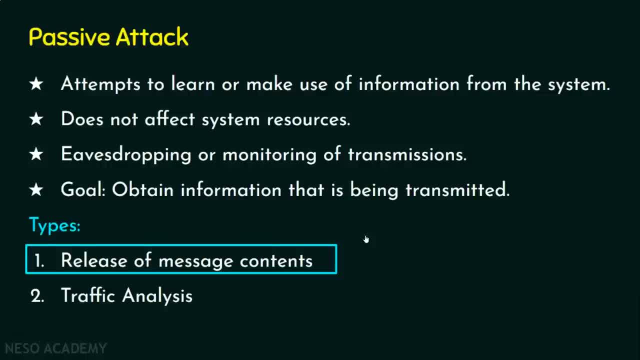 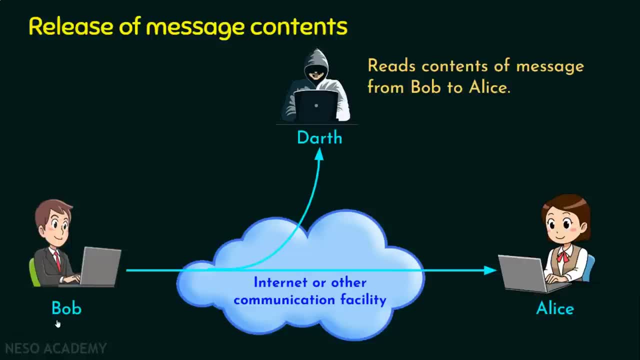 from the transmitter. We will see the first example: the release of message content In cryptography. we have two important characters that i would like to introduce. one is Alice and the other one is Bob. We consider Alice and Bob are the legitimate guys In this example. we consider this dearth to be an attacker. 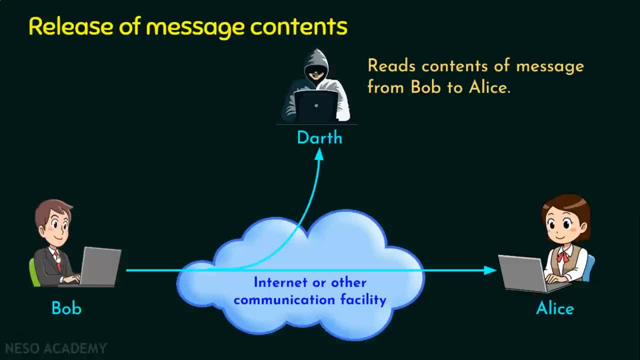 Now what is this release of message content? Say Bob is sending some message to Alice, so somehow Bob and Alice are connected to each other. it may be through the internet or any other communication facility. whatever message Bob is sending to Alice, Darth is getting a copy of the message. 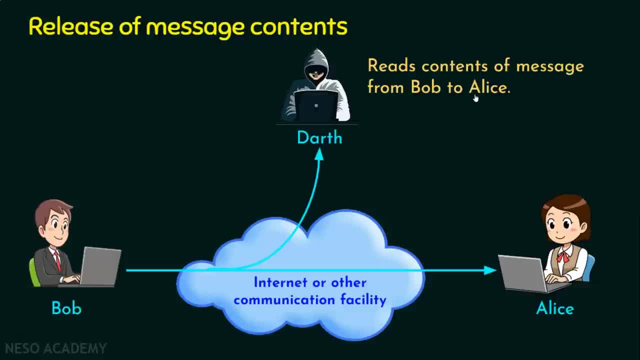 He is reading the contents of the message which is sent from Bob to Alice. So what Darth is going to do is Darth is going to understand or know what is the data that is being transmitted between the sender and the receiver. In this case, Bob is the sender. 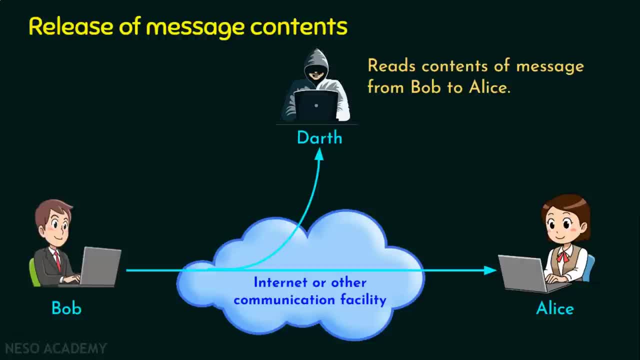 and Alice is the receiver. If Bob and Alice are exchanging information, if Darth is able to see the conversation, how to restrict this or how to prevent this? If Bob is encrypting the data before sending the data as such and Alice alone can decrypt, 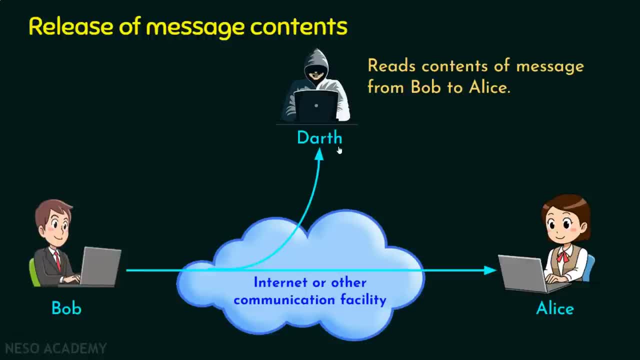 then Darth will have no way to see what message is being transmitted. But if the messages are not encrypted, obviously Darth will be able to know what is the data that is being communicated between the sender and the receiver. So we are done with the release of message content. 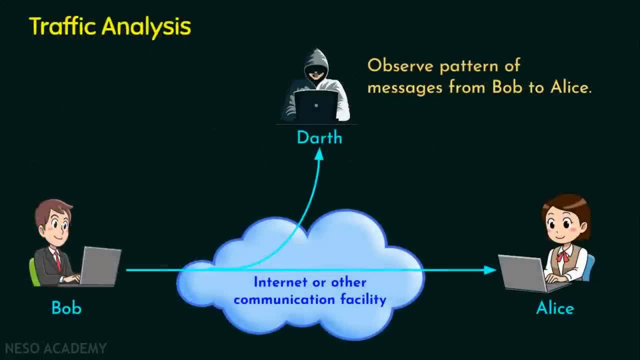 Let's now move on to traffic analysis. In the traffic analysis we have the same example where we have Bob to be the sender and we have Alice to be the sender And we have Darth who is the attacker here. Let's assume Bob has realized that. 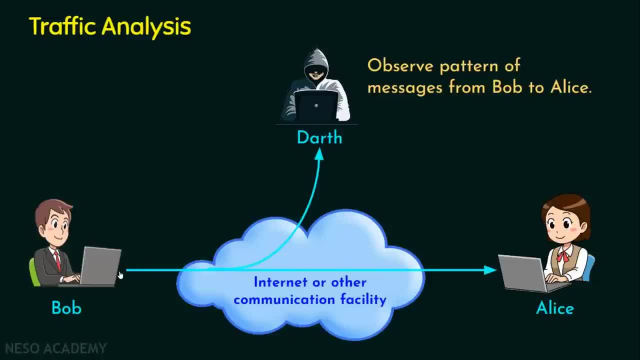 somebody may sniff the conversation or somebody may eavesdrop the conversation. What Bob and Alice have decided They have decided to do: encryption before transmitting the data. Let's assume in this example Bob is sending some encrypted data to Alice. Only Bob and Alice can understand. 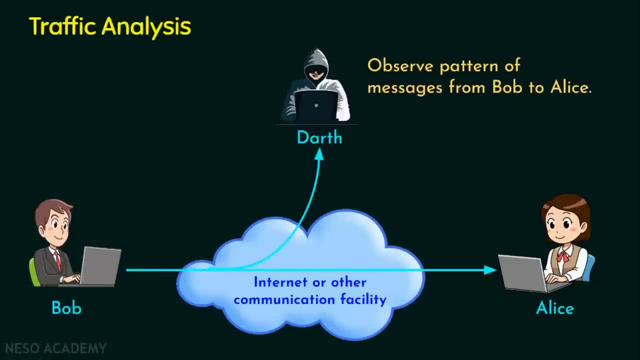 what data is being transmitted, because the data is now encrypted. The message is now encrypted. If Darth receives this encrypted message, he will be definitely not be able to understand what is the data. But still few information can be extracted like the location or the identity. 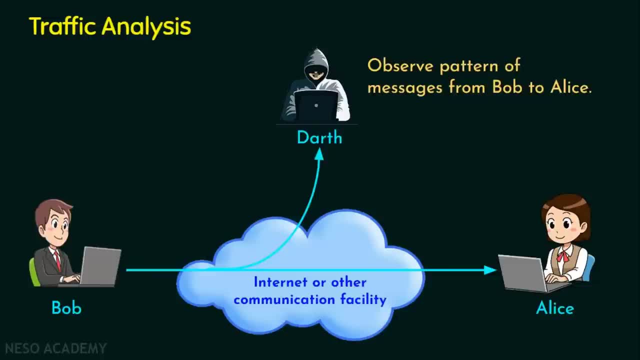 of the communicating host or the length of the message that is being transmitted between Bob and Alice, the frequency of message transfers between Bob and Alice. This information will be useful in guessing the nature of the communication that is taking place between Bob and Alice. So Darth will come to know about. 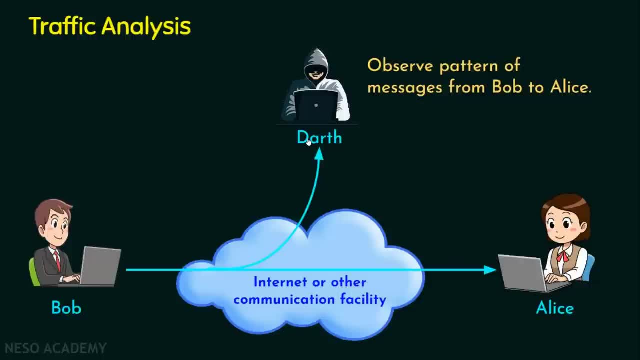 some information or Darth can guess what is the data that is being transmitted or what kind of data is being transmitted based on the traffic. So in traffic analysis Darth is going to observe the pattern of messages from Bob to Alice. We are done with passive attack. 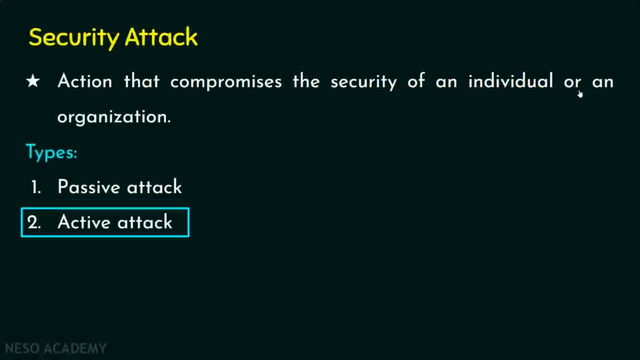 Let's now move on to active attack. We know in passive attack there is no modification of messages involved, just reading the messages, Whereas in active attack the active attack involves some modification of data streams or the creation of false data stream. Just recollect in passive attack. 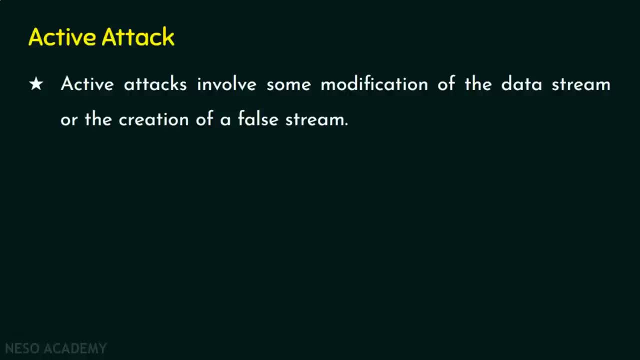 there is no modification of messages, Only reading of messages. So the attacker will be reading either the message or the nature of message that is being transmitted, if it is encrypted, Whereas in active attack, this active attack involves modification of the data streams or creation or insertion of a new data stream. 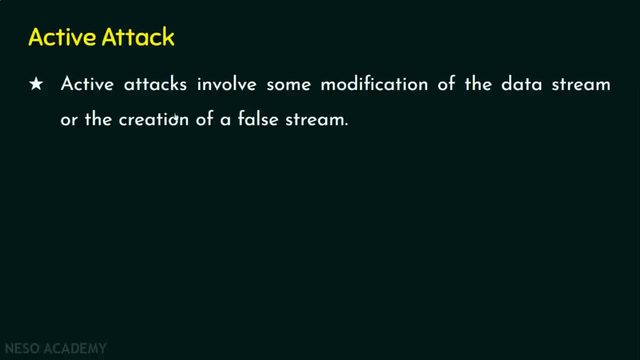 or a false data stream into the network. So active attack involves some modification of the message or the data stream. Basically, this active attack is subdivided into four categories: 1. Masquerade. 2. Modification of messages. 3. Modification of messages. 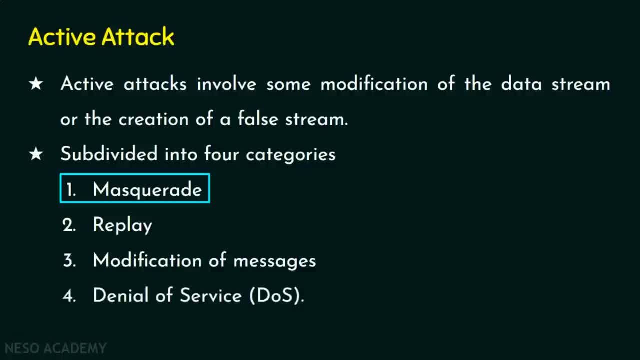 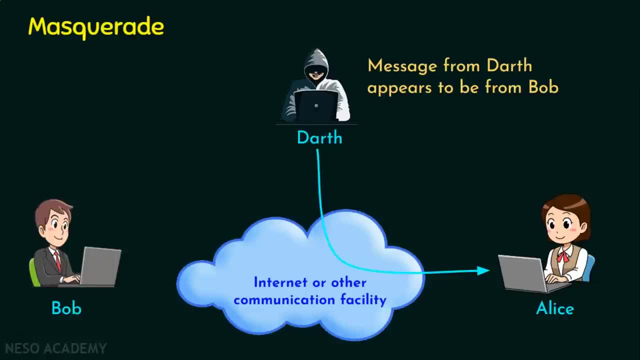 4. Denial of service. Let's start with the first active attack: the masquerade. What is this masquerade? In masquerade, one entity pretends to be a different entity. Suppose if I steal someone's username. 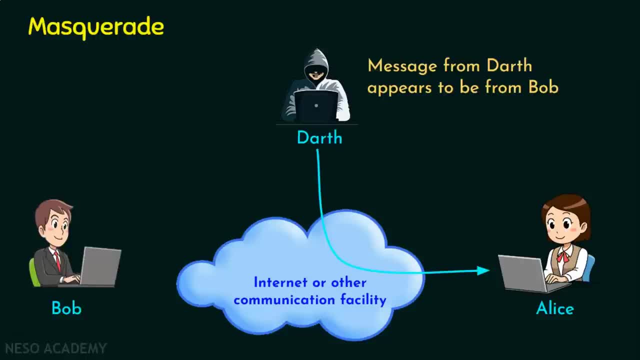 and password. and if I login with that username and password, I am a masquerader, Because I am not using my own credentials to login to the system. Rather, I am using someone's credentials to access the information What the system will think if I provide. 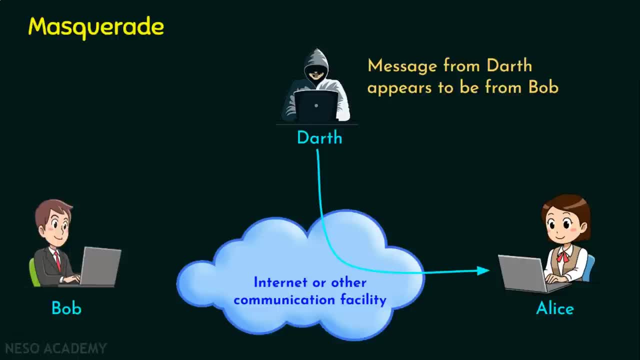 the username and password of somebody else, The system will think that that person only is using the username and password, Because there is no way for the system to ensure that who is using It verifies the credentials and provides the access. This is exactly masquerading is. 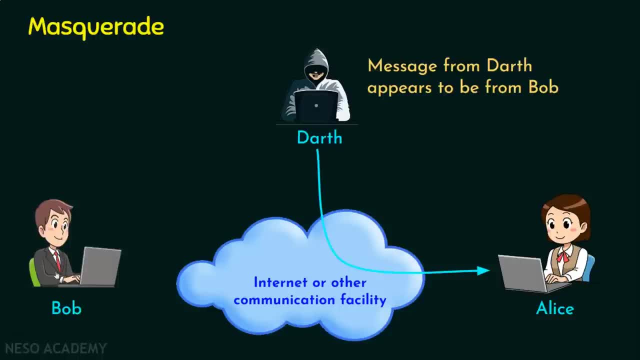 Previously, Bob only was actually communicating with Alice. So in this example, Bob is not sending any data transfer to Alice. Rather, Darth is sending some data to Alice. What is the attack here, then? Alice pretends to be Bob, So the message is what Darth is sending. 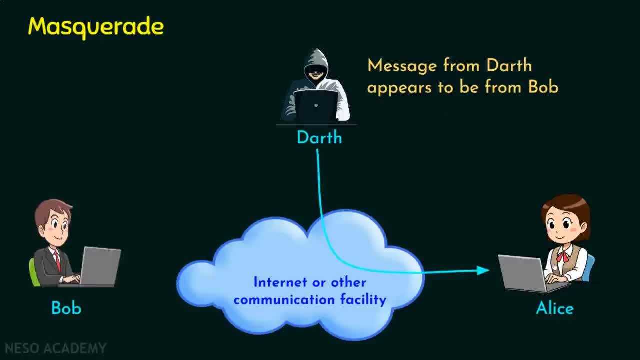 You know, the message from Darth appears to be from Bob. When Alice receives the message, Alice thinks that the message is from Bob, But actually it is from Darth, and Darth sends the message like Bob. This is exactly masquerading is. 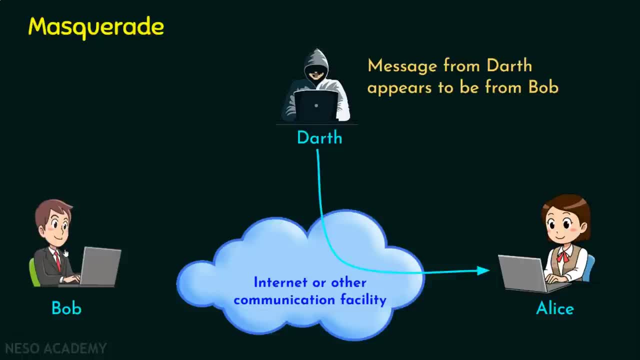 Then what we can achieve from this masquerading. Say, in this example there is an authorized entity. Let's take Bob as the authorized entity and let's assume that Bob is having few privileges only When he pretends like Bob. 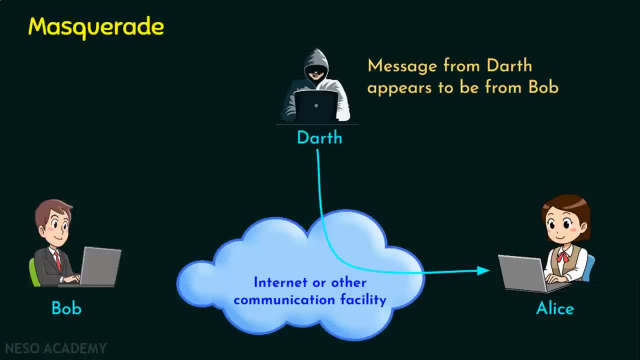 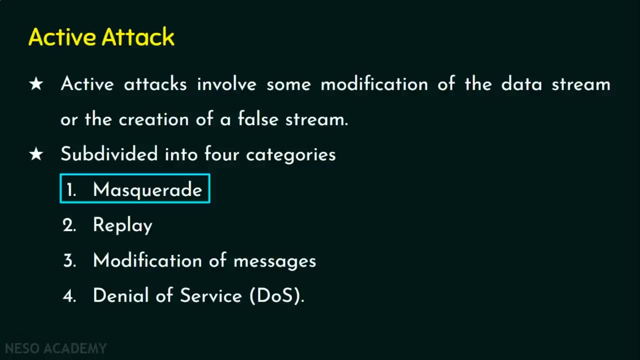 he may request some more privileges from Alice. So one example of this attack is an authorized entity with few privileges may demand for extra privileges. We are done with masquerading the first active attack. Let's now navigate to the second active attack. 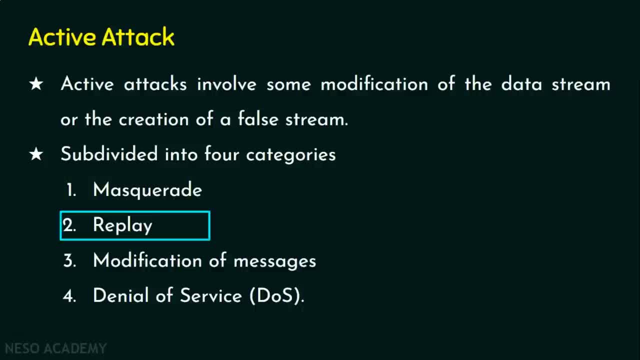 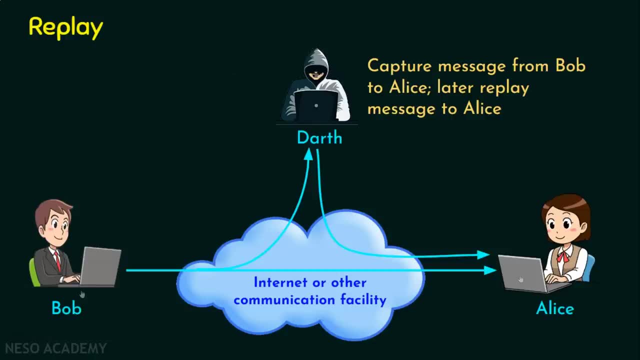 the replay attack. In replay attack the name itself says that there is going to be a replay activity, So the messages are subsequently retransmitted. So in this example can you see Bob is sending some message to Alice and here done. 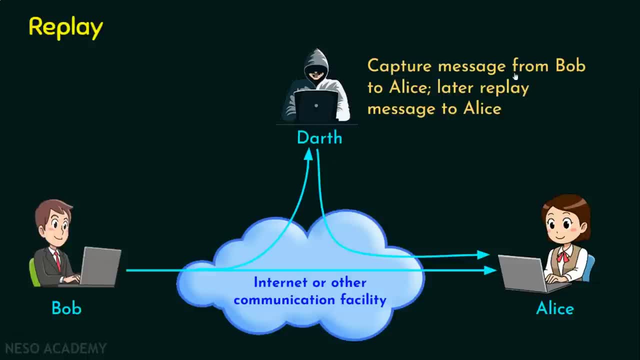 Darth is the attacker. What Darth is going to do? Darth is going to capture message from Bob to Alice and later replay the message to Alice. Say, for example, Bob is sending some data items to Alice and Darth is going to collect all the messages. 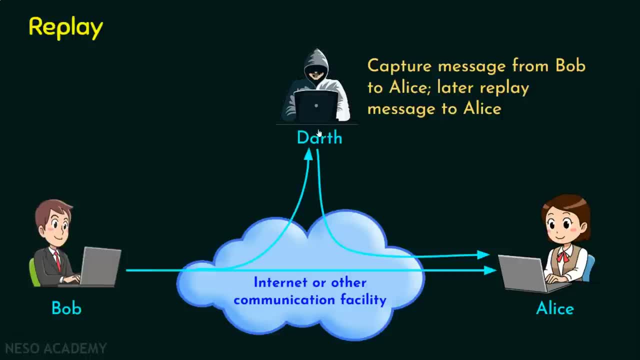 which is sent by Bob to Alice and later Darth is going to replay or send the same messages subsequently, again and again in order to provide an unauthorized effect so that Alice will be confused and provoked. This is replay attack. We are done with the second type of active attack. 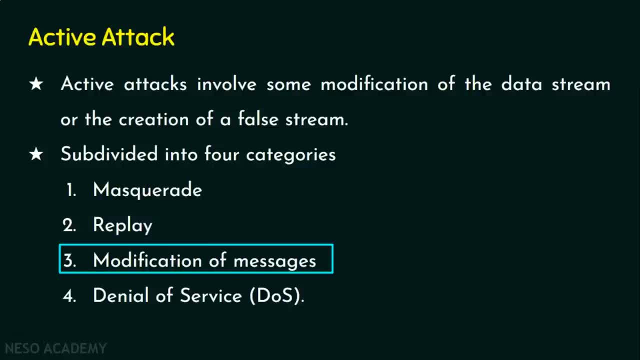 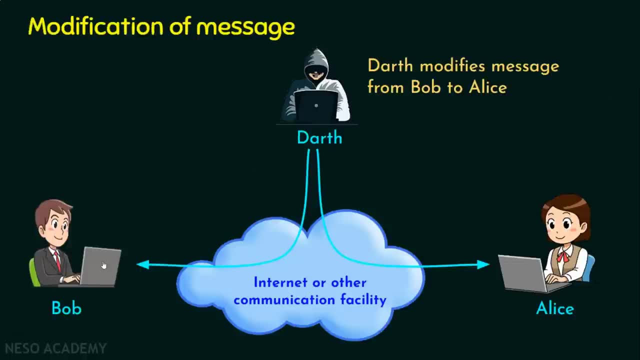 The replay attack. Let's now move on to the third type, which is the modification of messages. So the name itself says that the messages are going to be modified. Let's see an example. In this example, Bob is going to send some data to Alice. 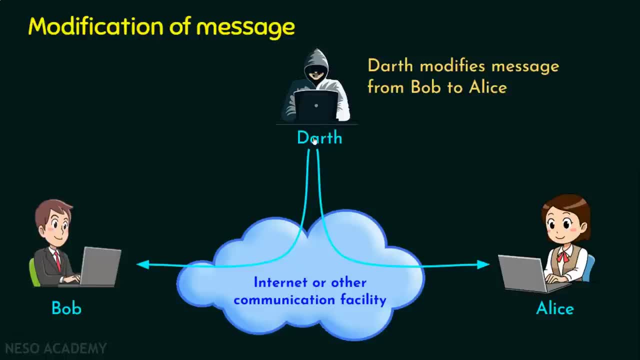 So Bob is going to send some data but Darth captures the message Later. Darth, after capturing the message, is going to modify the message and send that message to Alice. Now Alice receives the modified message, not the original message which was sent by Bob. 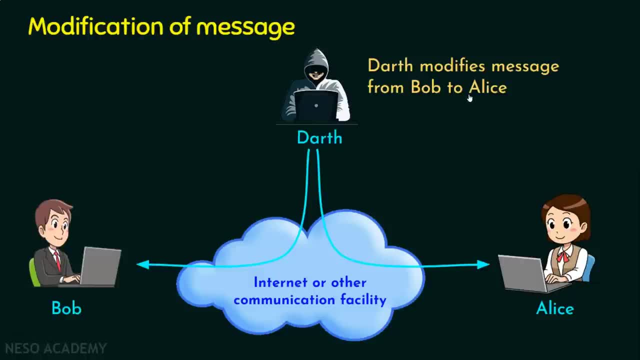 So that attacker Darth here modifies the message from Bob to Alice Say, for example: if Alice is sending a text, Allow John to edit the document. What Darth can do? He can capture the message, He can modify the original message. The original message is: 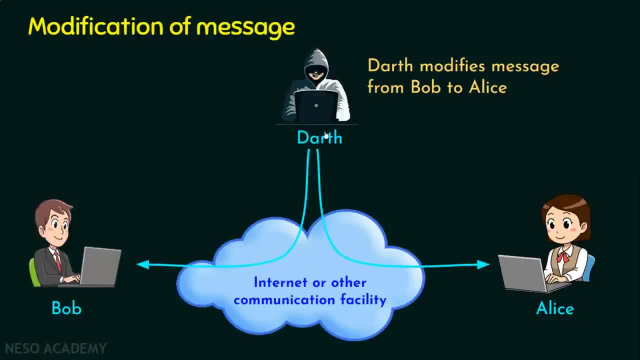 Allow John to edit the document. But what Darth is going to do? He is going to modify the message. Let's assume instead of John he is placing the word Tim. So now what Darth is going to send to Alice? Allow Tim to edit the document. 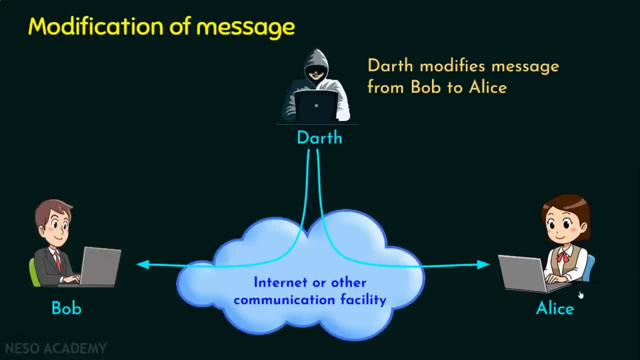 Bob created the text. Allow John to edit the document. What Alice is receiving. Allow Tim to edit the document. So this is also an attack. This attack we will call as modification of messages. We are done with the third type of attack. 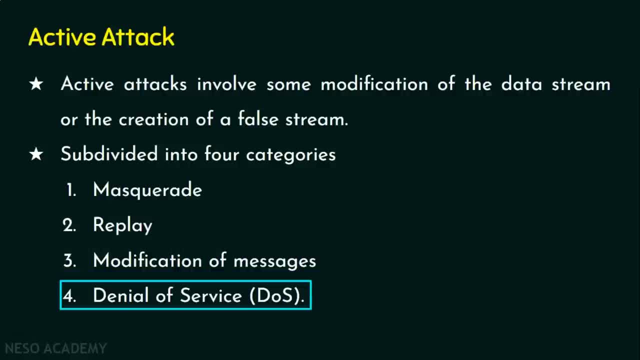 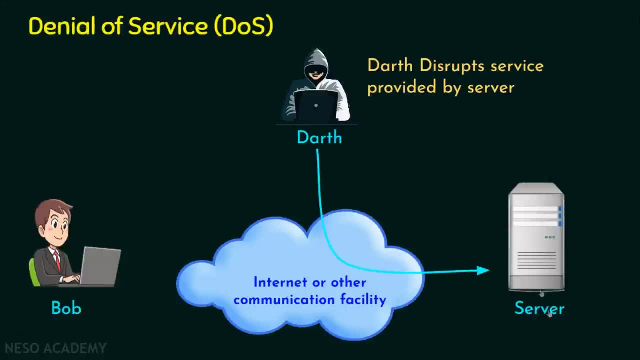 which is the modification of messages. Let's now move on to the fourth type, The last type, the denial of service attack. The name itself says that we are going to be denied from getting the service. Let's see an example. In this example, Bob wants to access the server. 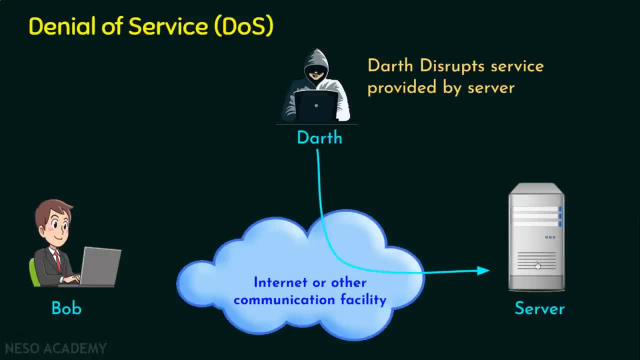 But what Darth is going to do? He is going to do some activity or action on the server such that Bob is getting denied from accessing or getting the service. Bob is actually in a need of getting service from the server, But what Darth is doing? 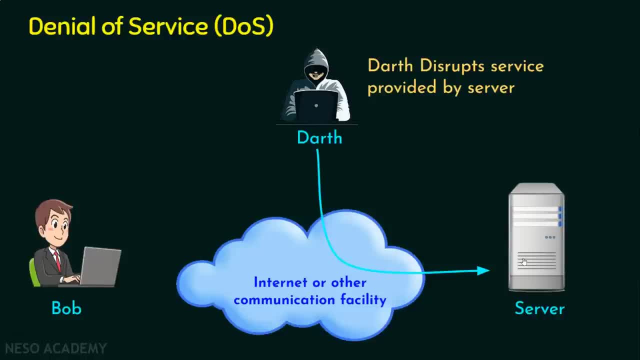 Darth is overloading the server, or Darth is putting a lot of stress on the server in such a way that the performance of the server is degraded and the server is no more able to service new clients. So when Darth wants to access the server, 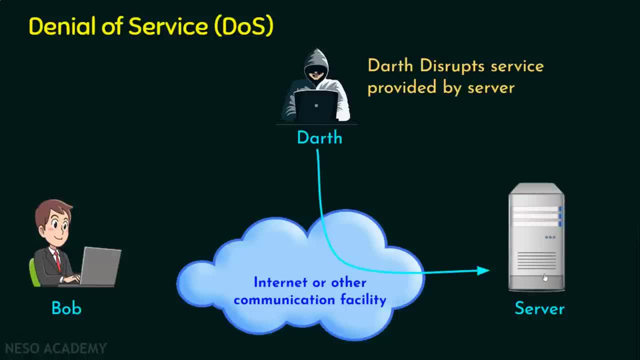 the server is already overloaded and the server cannot consider the request of Bob, So Bob will not be getting the service. Now Bob is getting denied from getting the service. Now Bob is getting denied from getting the service. This is denial of service attack. 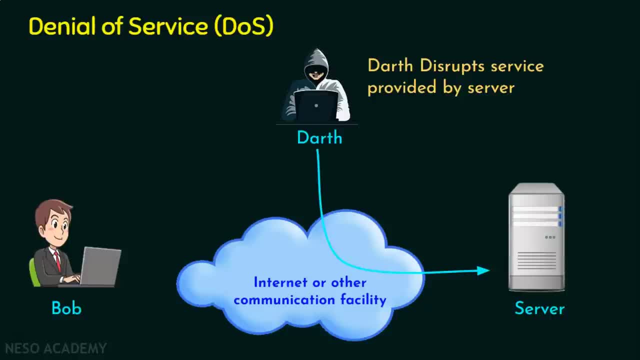 See, basically there are multiple denial of service attacks. See, basically there are multiple denial of service attacks In computer network lecture series. I told you, before any communication takes place in TCP, the connection establishment phase will be the first phase, right, 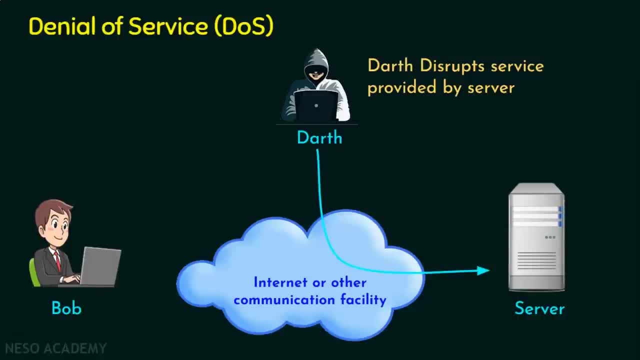 So before data transfer, that can take place, connection establishment: the three-way handshaking will be performed. What if Darth is creating a malicious program or a bot program in his system and a lot of data transfer and a lot of TCP connections are established with the server. 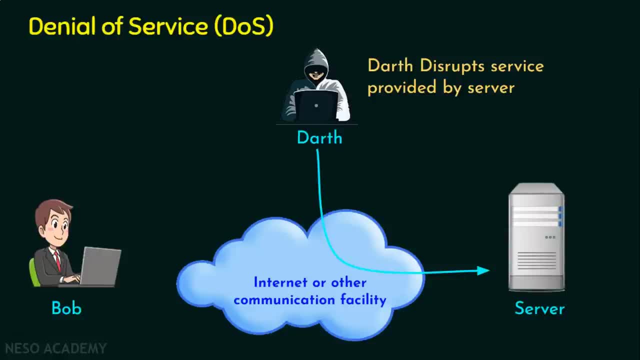 I already told you, attackers are intelligent guys. So how Darth is going to create this malicious program? you know he is going to create a program in such a way that from his computer a lot of TCP connection request is going to reach server. 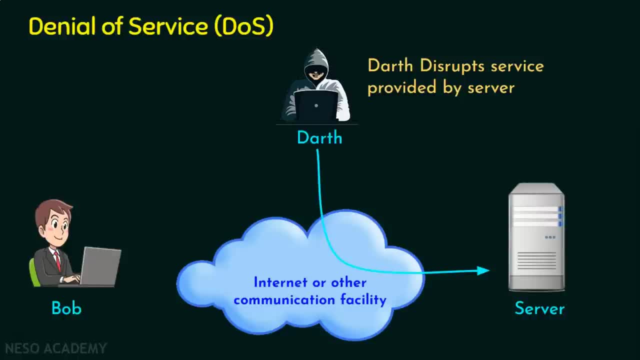 but the server will be thinking that it is from different computers In real time. we have a lot of tools to launch denial of service attacks, but never try denial of service attacks without the knowledge of the owners. According to the server, server thinks that 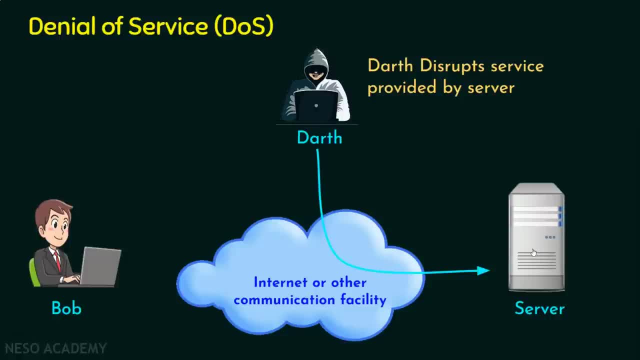 there are different clients, So at one fine point of time the server becomes overloaded with a lot of requests. So obviously Bob will not be able to access the server, right? This is denial of service attack. There are multiple denial of service attacks. 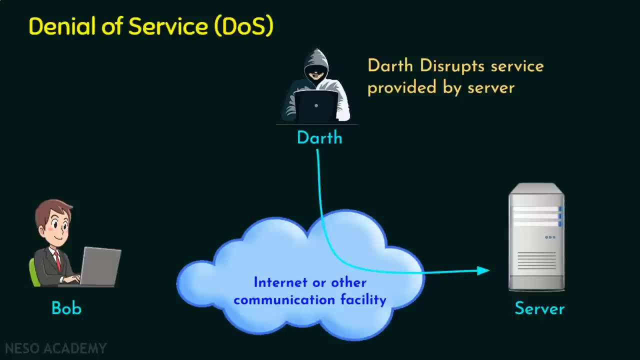 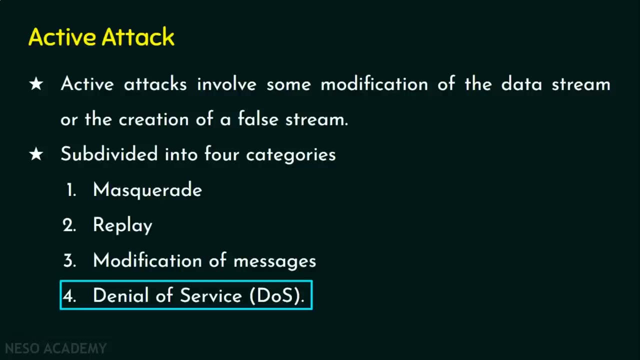 In this example we have seen the TCP connection establishment way of denial of service attack. There are multiple denial of service attack exist in today's world. That's it. we are done with the fourth type, the denial of service attack. So we are done with the active attack also. 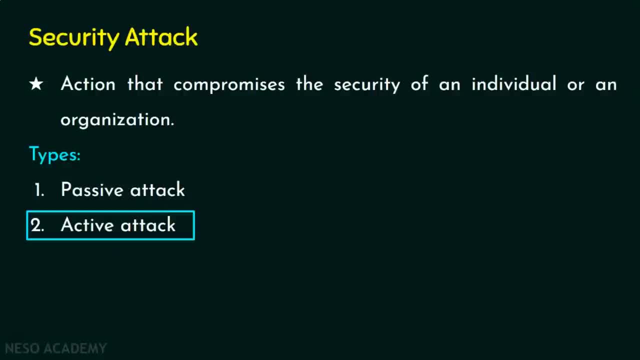 Before we conclude, let's see the difference between active and passive attacks. We know the basic difference between the passive and active attack. Passive attack will not involve in modification of messages, whereas active attack leads to modifications of messages that is being transmitted. Let's start with the passive attack now. 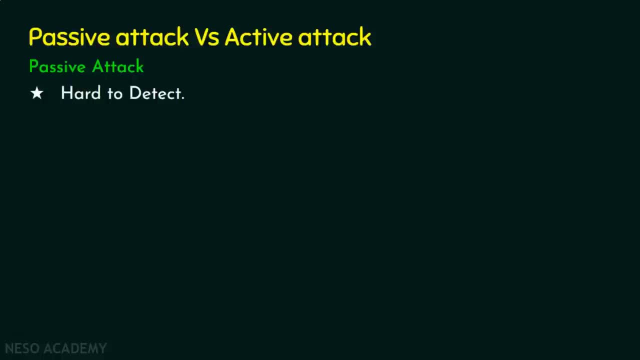 Generally, passive attacks are hard to detect because there is no modification of the message involved. If the messages are modified, we can verify whether the message is modified or not, But passive attacks are just reading or eavesdropping the conversation. How many people have read the conversation? 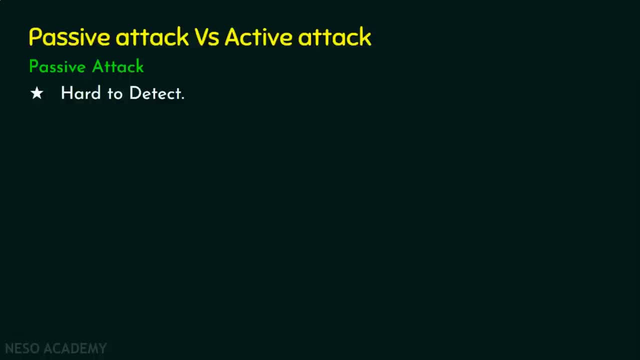 Say you want to send a letter to your friend and before the letter reaches your friend, let's assume 10 people have read the message without modifying the message. How can you or your friend come to know how many people have read the message? 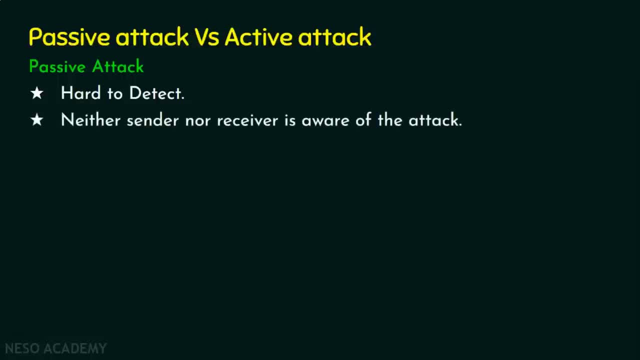 So that's practically not possible, right? So passive attacks are generally hard to detect and neither the sender nor receiver is aware of the attack, because the messages are not modified. And how to prevent passive attacks If the messages are sent as plain text? 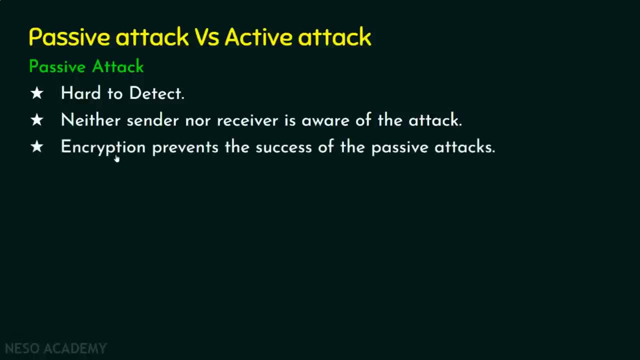 then it will be difficult to prevent, right? If the messages are encrypted, then except the sender and receiver, no one can understand what the messages are. right? So encryption prevents the success of the passive attacks. As far as passive attack is concerned. 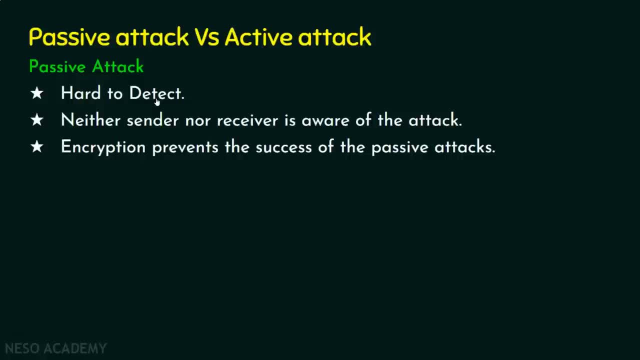 we know detecting the passive attack is very hard. So what should we do? We should focus more on preventing the passive attack. So in passive attack more emphasis is on prevention than detection. And coming to the next attack, the active attack, 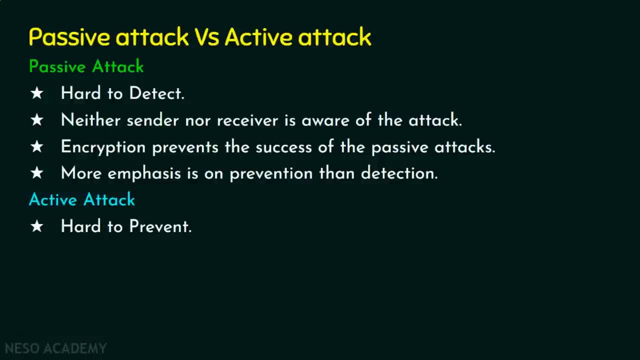 So generally active attacks are hard to prevent because we can't prevent the attacks and we can't easily detect the attacks because there will be modification of messages, As mentioned. it is difficult to prevent. So there are chances for the physical or the software or network vulnerabilities. 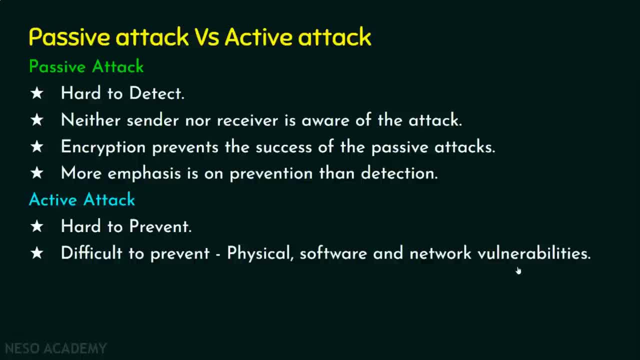 to take place. This active attack may involve in the physical devices or in the software or in the data that is being transmitted, or maybe in the network as well. Whenever there is an active attack, we must detect and recover from any disruption or delays. 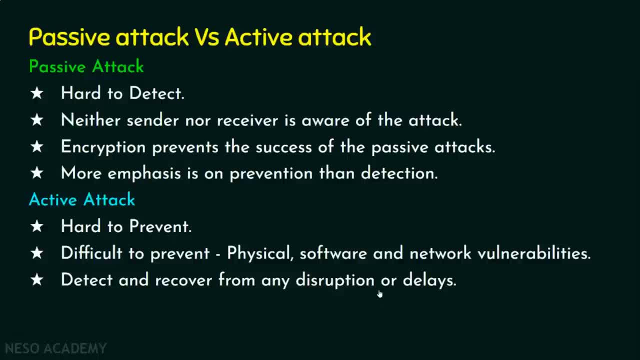 We need to immediately act upon it, Otherwise there could be a disaster in the organization As and when the active attack is detected. we need to detect and recover from any disruption or delays of the service, because it is more important right And finally, if the detection has a deterrent effect. 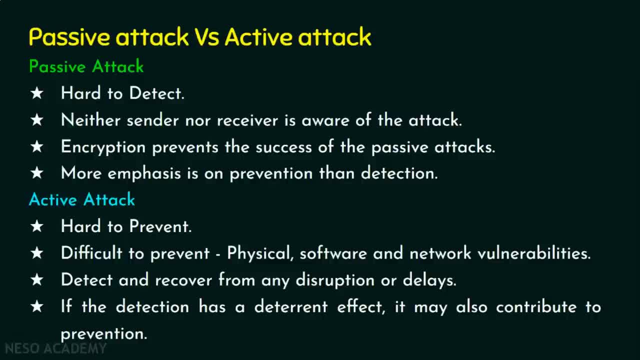 it may also contribute to prevention. So we should focus on detecting as well as preventing the active attack. Now I will just put a question this way: Which attack is more dangerous? Is it passive or active? I know many people will answer. 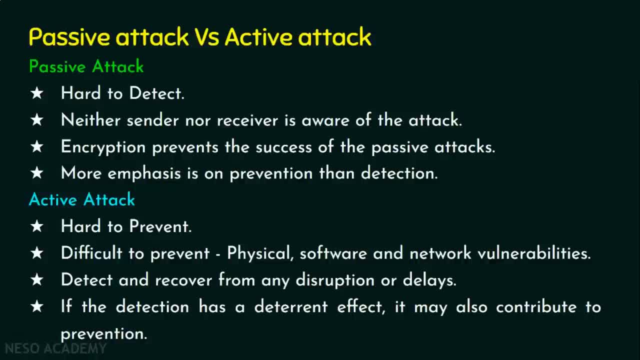 active attacks are more dangerous. I will tell you both the attacks are dangerous because a confidential information breach or the security information breach, let's assume- a confidential information maintained by an organization, maybe it's customer's record or payroll information or any other sensitive and highly confidential. 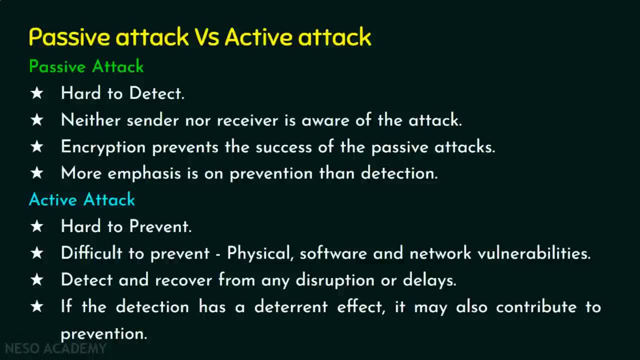 information by that organization, or even a government related information, which is considered to be the most confidential data, or military related data. if it is passively attacked, no modification just revealed, it leads to disasters as well. right, Both the attacks are dangerous.